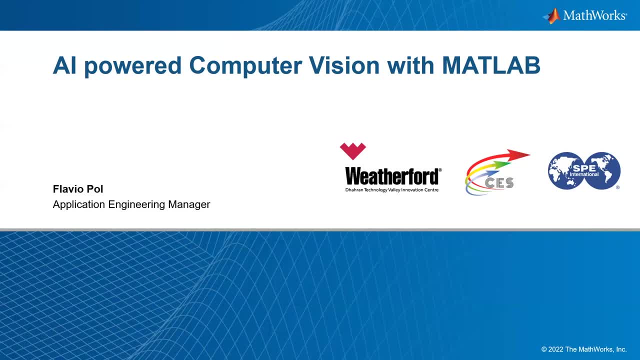 we can get and explore this interdisciplinary scientific field of computer vision. In this webinar, I will explore computer vision toolbox algorithm, functions and apps for designing and testing computer vision systems for feature detection, extraction and matching. In addition, we will also explore how to train customize computer vision AI models using deep learning. 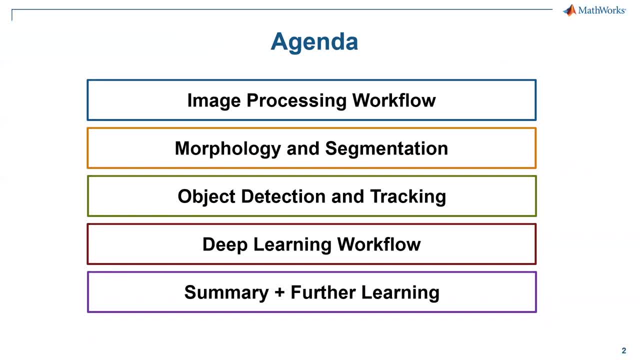 This is our agenda for today. So first we will introduce image processing workflow, After we're going to jump to morphology, and segmentation are very important. It's very important to understand morphology segmentation because there are some operations that are essential for the computer vision capability, Because it's very important for 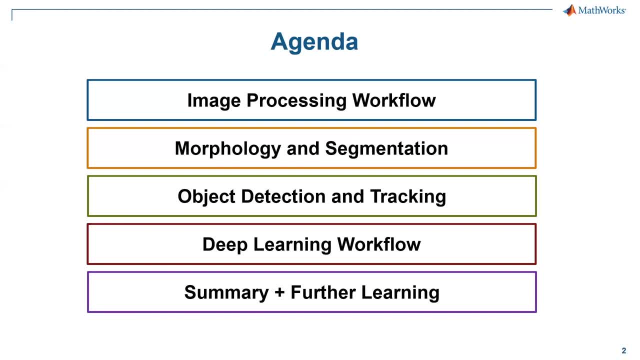 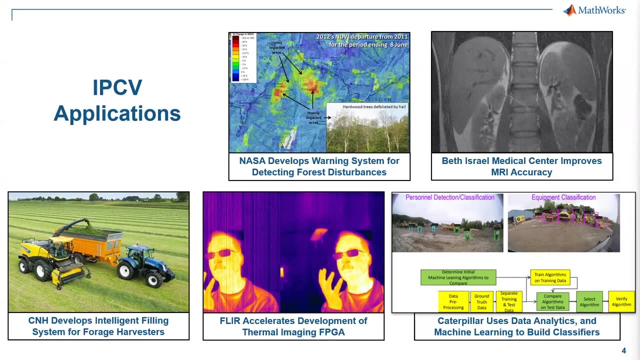 the computer vision applications. So, after we're going to jump to object detection and tracking and deep learning workflow and we're going to finish with a summary and how you can explore more about computer vision in MATLAB, This is some applications in image processing, computer vision, that are in the website So you can explore and see what. what is the problem, how it was solved. 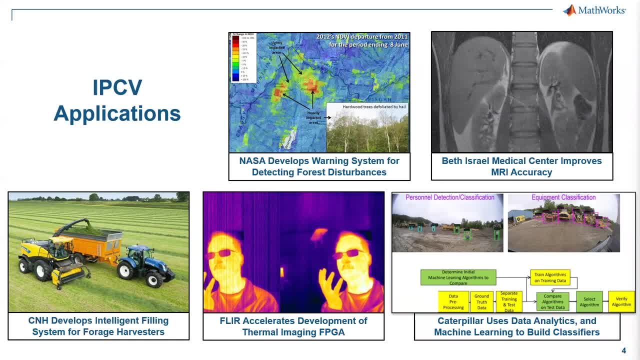 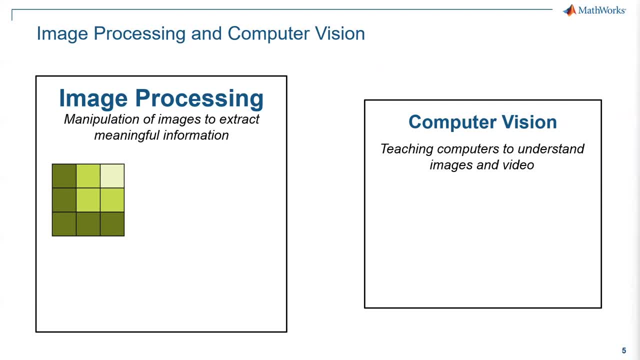 and also the what the company accomplished with this workflow. So here is a very quick introduction to image processing and computer vision. The two domains go hand in hand. In image processing is often done prior to computer vision to learn something about the image. So here you do some thresholding and after you understand you can. 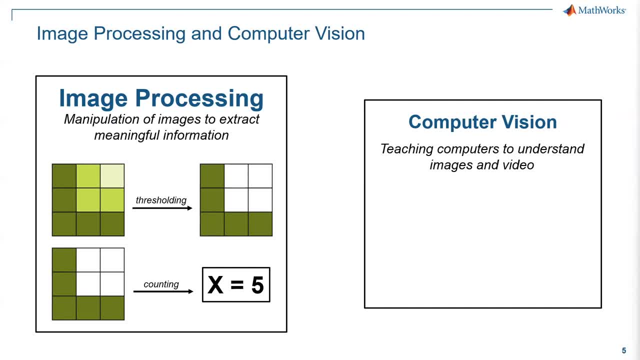 count how many pixels are in the in the image. So image processing is about a manipulation of image to extract meaningful information, such as counting number of pixels in an image. However, computer vision is about understanding image, or teaching computers to understand images such as this is a letter L.